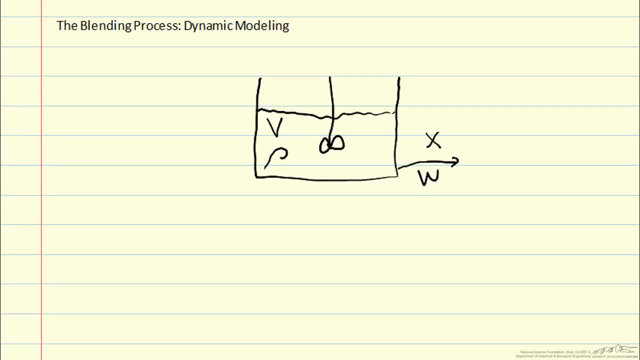 but it will also have a density- rho, that we will assume is constant. We will assume that we have liquid in the tank which is incompressible and that the species A of interest is dilute such that its amount doesn't really change the overall density. 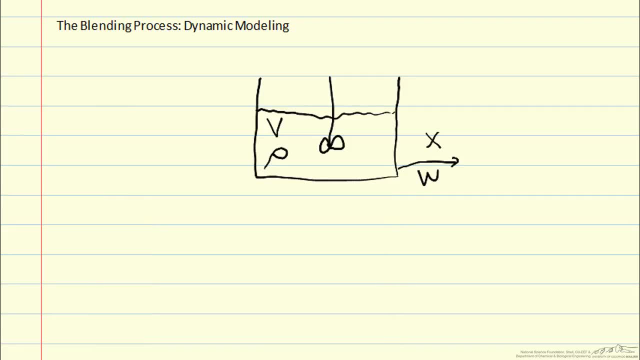 This is the blending process and we are going to blend two streams coming in: Stream 1 that has mass fraction X1 and flow rate W1.. We're going to blend it with stream 2 that has mass fraction X2 and flow rate W1.. 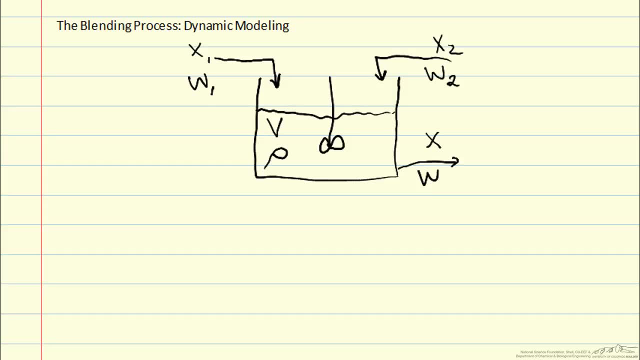 Now for this particular control problem. we are interested in controlling the mass fraction X. that is our control variable, or CV, and we're not going to be able to influence stream 1. That's coming from some upstream process, so that's our disturbance variable or DV. 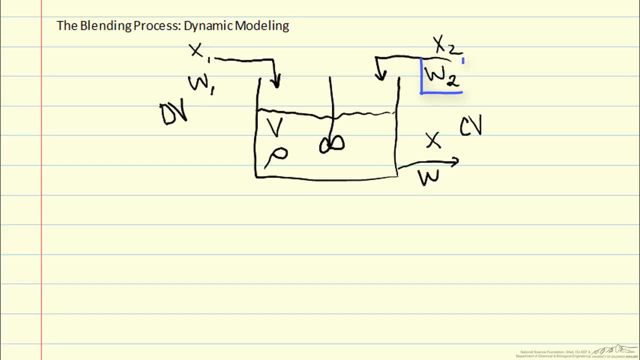 But we will use stream 2 to manipulate the process. W2, in particular the mass flow rate, will be our manipulated variable, Or MV, And we are going to build a dynamic model based on balance equations. Anytime you do that, you should really carefully describe your control volume. 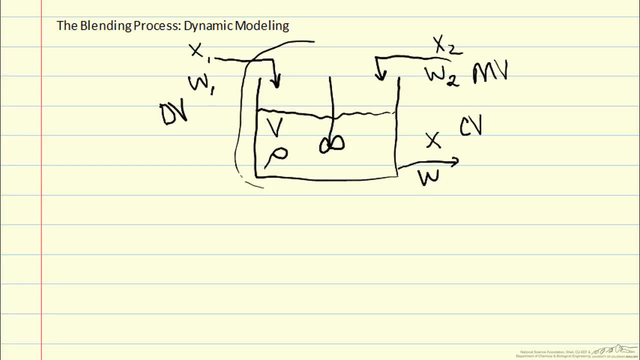 So that you know what is going in and what is leaving the control volume, So that you know what to balance. So here we'll draw our control volume And we're going to use balance equations to construct our dynamic model. Usually we balance either mass or energy. 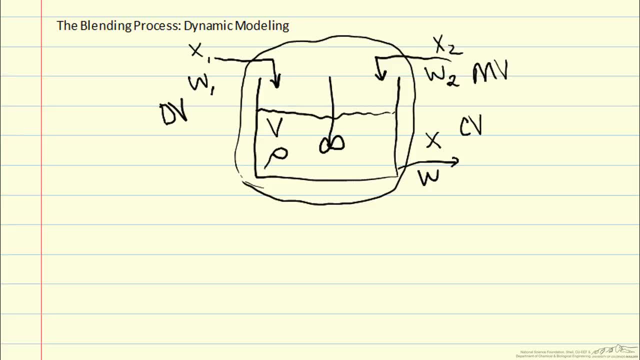 And here we were not given any information about energy, No temperatures or heat flows, But we were given mass flows. So let's go ahead and construct a mass balance. First we will consider the mass in the entire system, So the total mass here. 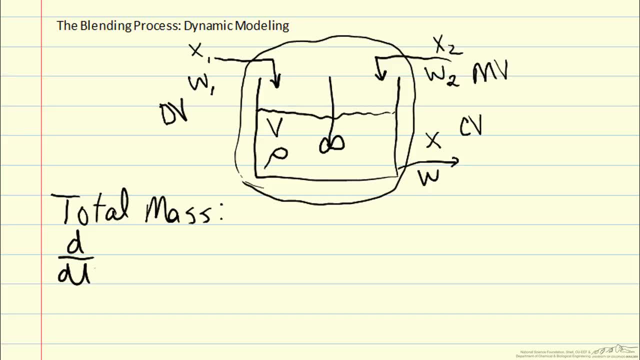 So let's look at the accumulation in the control volume of mass. So accumulation is equal to what is going in W1.. W1 plus W2. Minus what is leaving, And we can break down that mass variable into variables that we used in our diagram above. 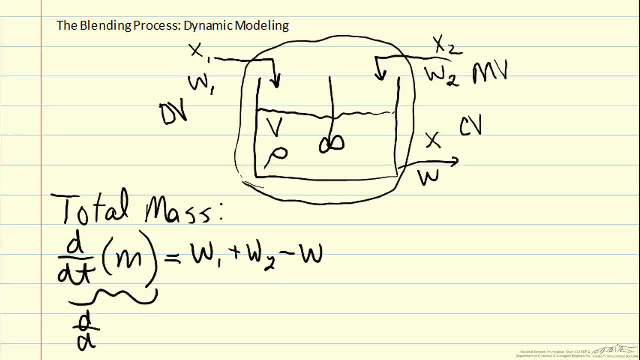 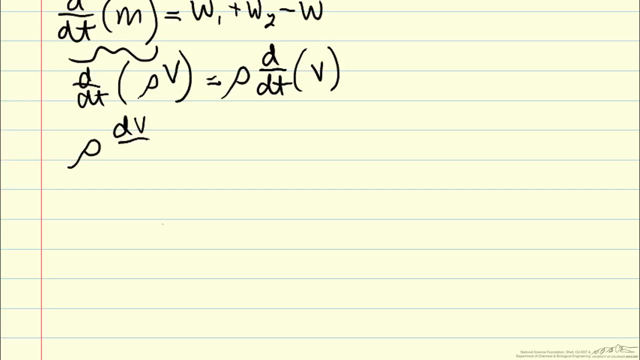 So in particular, we can break that down into d? dt of rho times V, Density times volume, And because density was assumed to be constant, we can pull it out Of the time derivative And we just have volume inside now. So now we can write our total mass equation as rho. 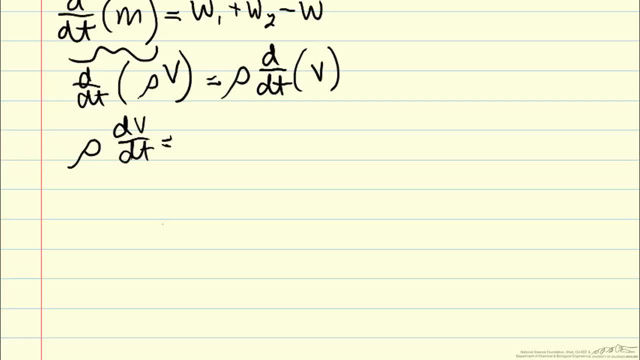 dv. dt Equals W1.. Plus W2.. Minus W. Now this will tell us about how volume changed, Which is depending on flow rates in and out, But it doesn't tell us about our control variable, Our mass fraction x. 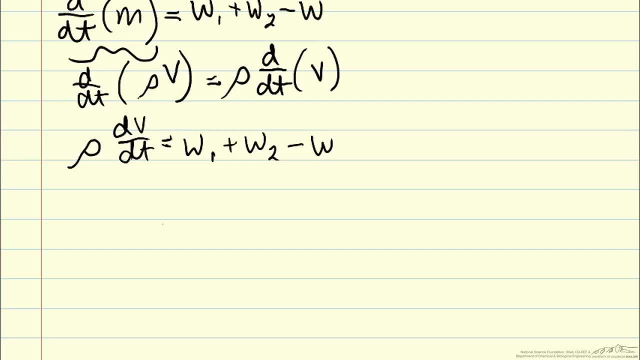 So, in order to describe x, which is the mass fraction of species A, We should perform a second balance On the mass Of A. So now, if we look at the accumulation of A in the control volume, That's the total mass. 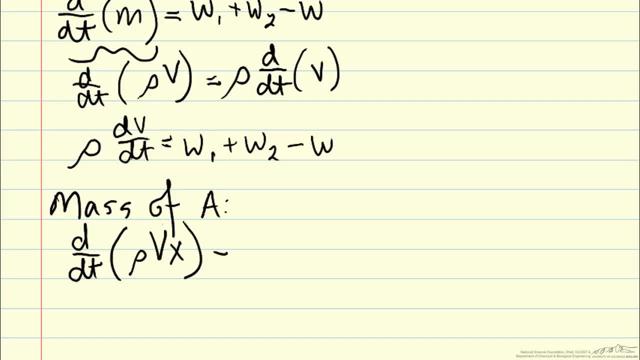 Rho V Times the mass fraction x, And that will be equal to The amount of A flowing in, Which is W1. X1. Plus W2. X2. Minus W, X, And again we can break down. 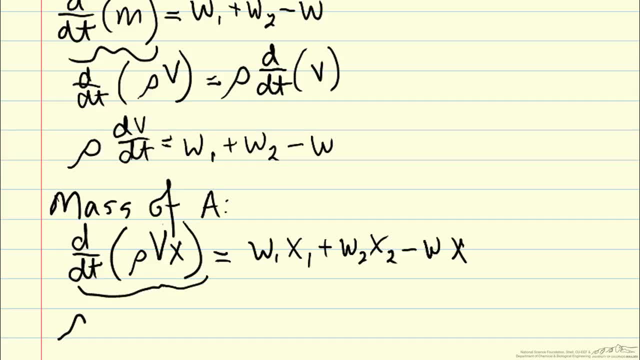 The mass of A By pulling out the rho. But now, Within our ddt term, We have two time varying quantities- Volume And mass fraction, So we'll need to use the product rule In order to break that down into our 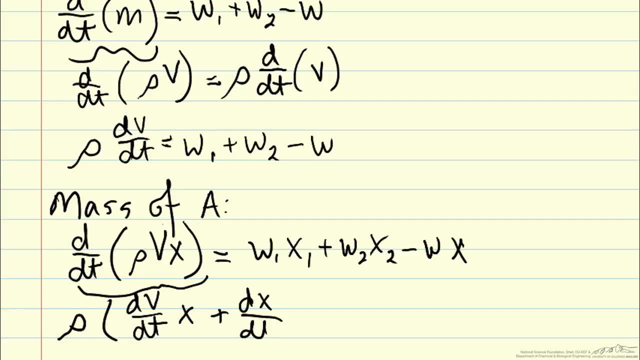 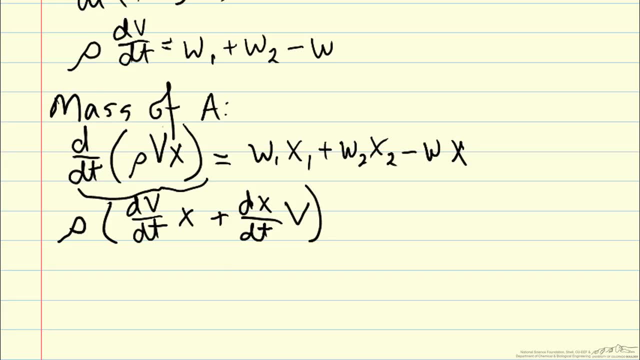 Two different variables, X and B. So be very careful When you're pulling terms out of your ddt. Make sure they're constant Before you pull them out of the ddt. So now we can write A balance equation, A dynamic equation. 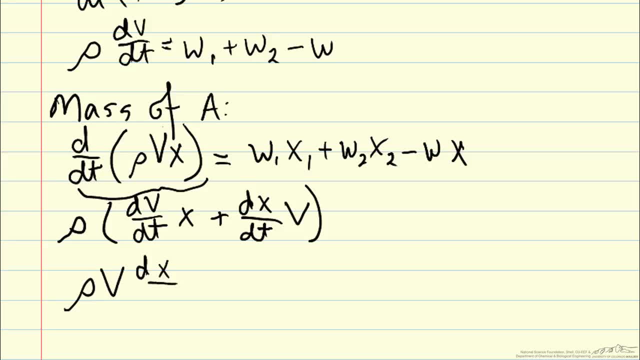 For dx dt. So we can write: Rho V, Dx Dt Equals W1. X1. Plus W2. X2. Minus Wx. And then we need to move that dvd term To the other side. 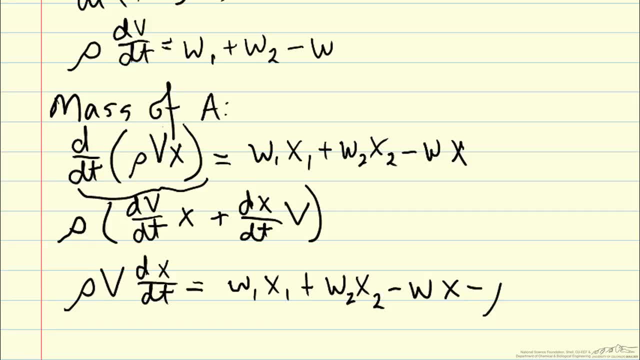 So we have Minus Rho, Times X, Times Dvdt. But we already know What is Rho Dvdt From our total mass Equation Up there at the top, So we can go ahead and plug that in.